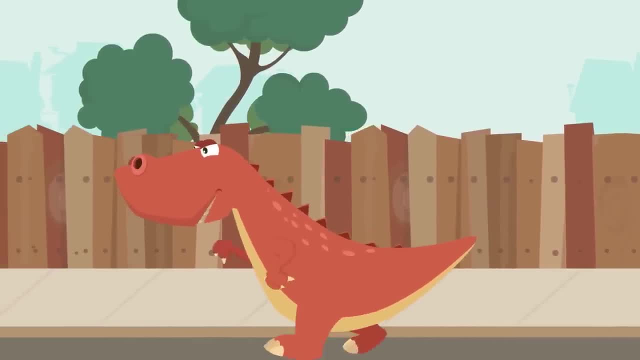 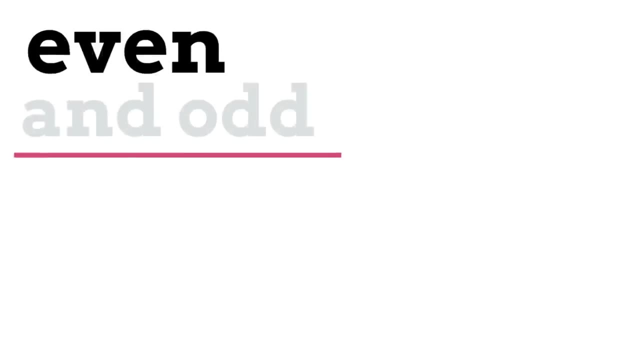 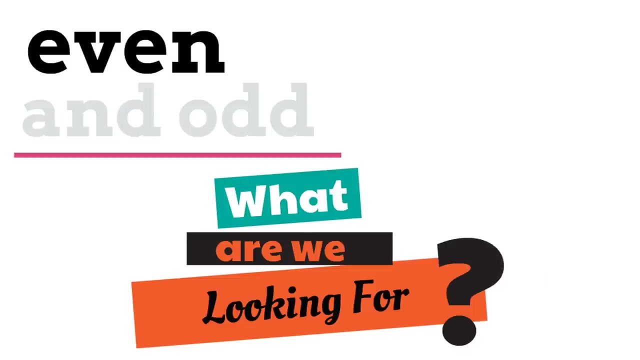 ready to help us discover the secret right To knowing even and odd. So what is this key that we're looking for? What are we looking for that will tell us if a number is even or if the number is odd. An even number. 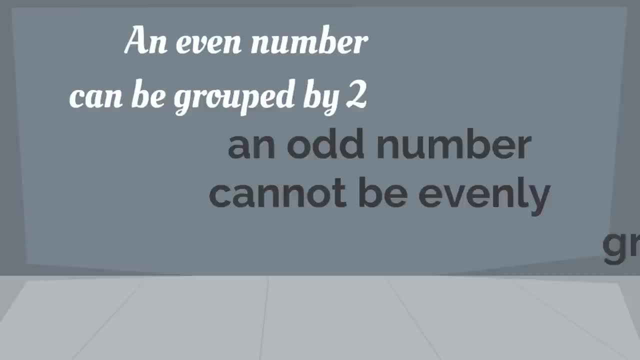 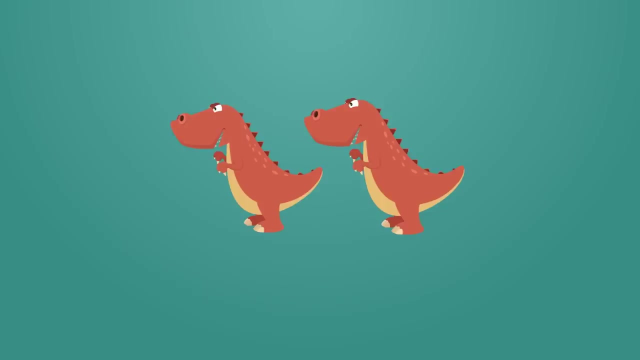 can be grouped by two. An odd number cannot be evenly grouped by two. So it's all about the number two and that might sound confusing. Let me show you and you'll see. Here is the easiest number to do. We're looking for the number two, okay. 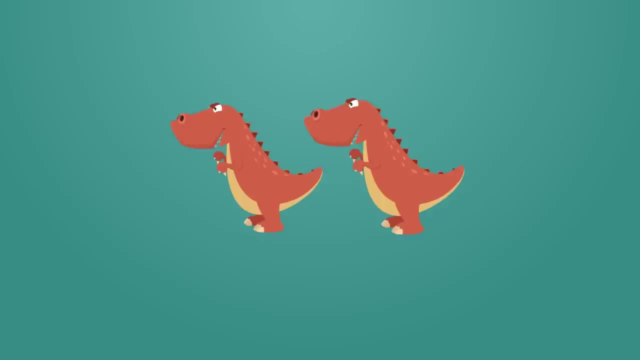 Can it be put in a group of two? Well, yes, because it's the number two. We've got two dinosaurs. That makes two. even Now, this is odd. This dinosaur is all alone. He's not in a group of two. This makes the number one. 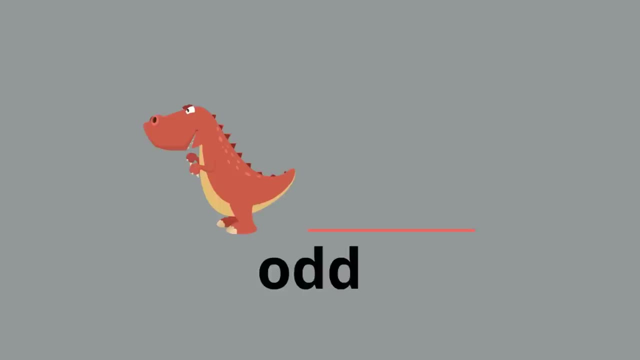 an odd number because he's all alone. That's odd, It's an odd number. Let's look back at the number two. See what's neat about this is it's an even group of two. That means our dinosaur has a friend. He can talk to his friend, He can hang out. It's. 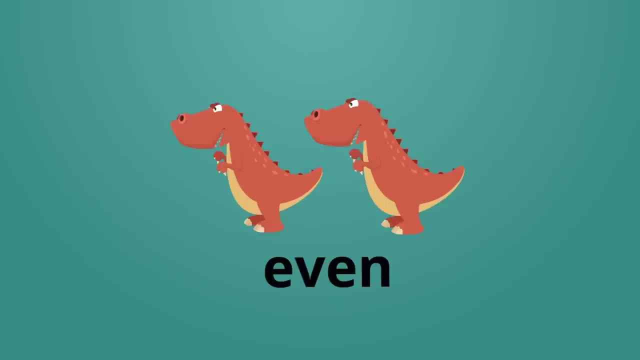 not, it's not weird, It's not odd, It's an even number. Here we have three dinosaurs. Now can we put the number three in even groups of two? Well, no, because that third dinosaur is all alone. The top two dinosaurs have somebody. Three is odd. 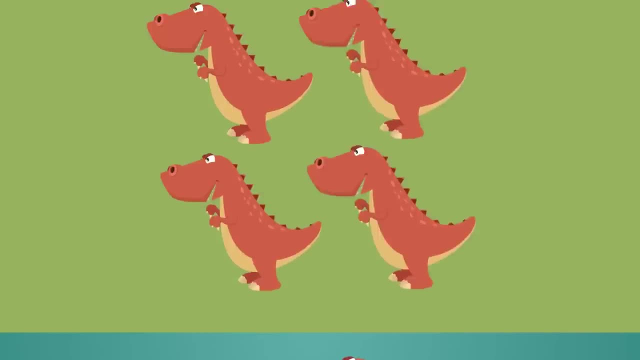 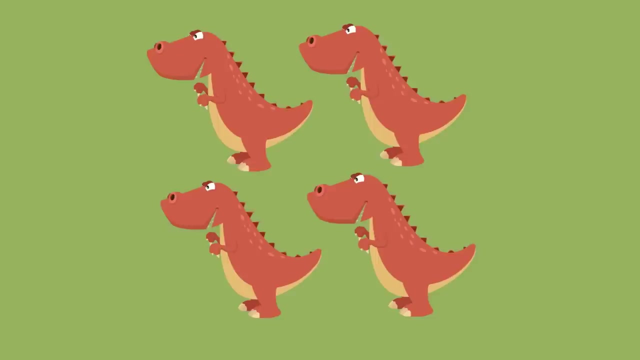 There's one that's missing a partner. Here we have four dinosaurs. Now we're looking for groups of the number two. Now we have two groups of two here. That means it's an even number. Each dinosaur has a friend. Wow, Five. 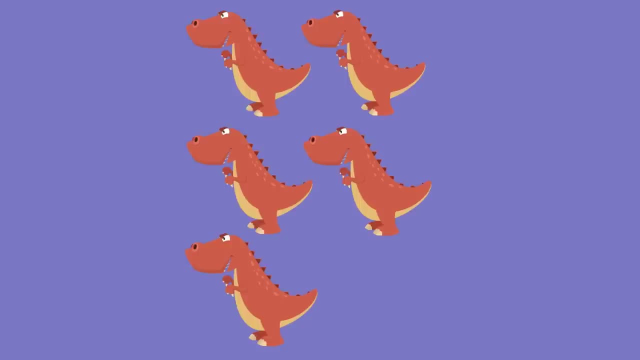 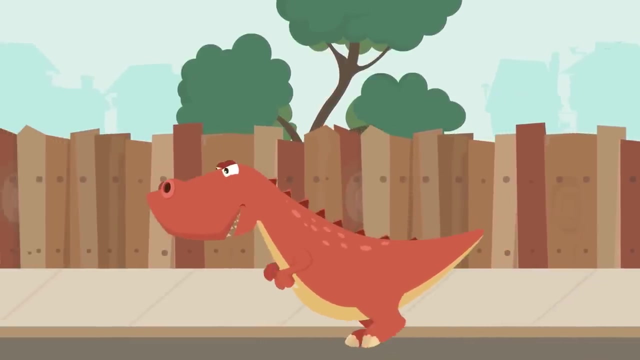 dinosaurs. But look, one on the bottom doesn't have a pal, doesn't have a friend. That's odd. It's not evenly grouped into two. Five is an odd number. Hey, buddy, okay, don't don't run. Okay, we'll get back to the even numbers. I know you don't like the odds, You don't. 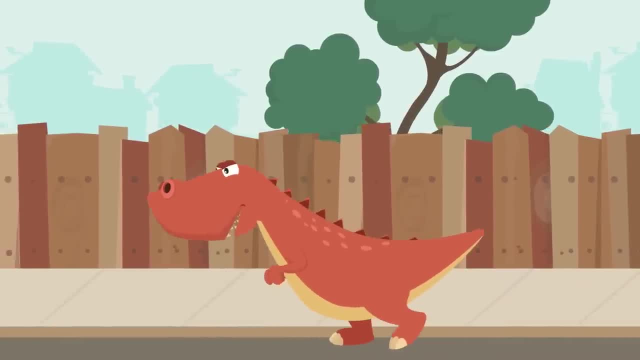 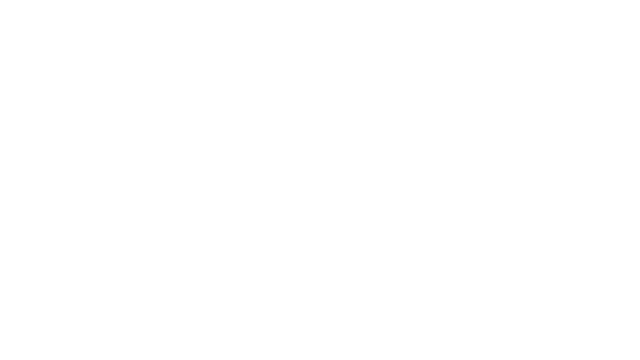 like being the odd dinosaur out, It's okay. I promise this next number is going to be even, because it goes for even odd, even odd. Just hang on. Oh man, Dinosaurs, You know so temperamental I mean. what's that all about? I mean a dog. 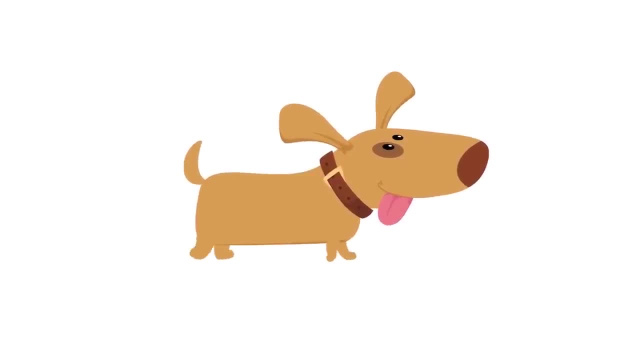 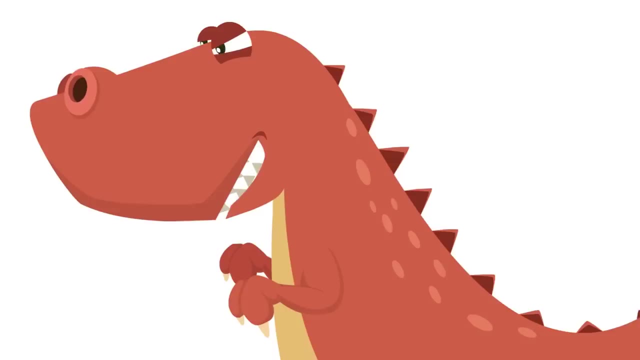 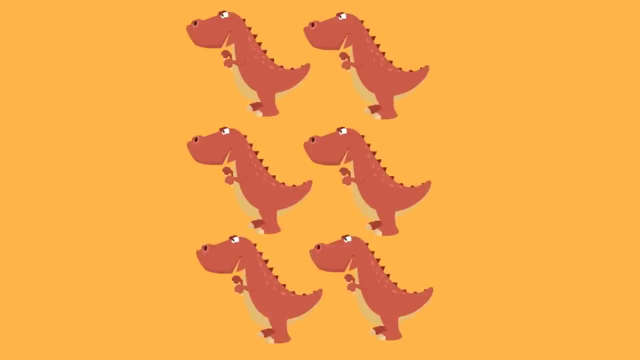 Dog wouldn't have done that. you know, Dogs are better, I think now, than dinosaurs. I'm just kidding, Dinosaurs are so cool. Moving on Here we have six dinosaurs Now. each dinosaur has a friend. that means six is even. you can split it up in groups of two. oh, here. 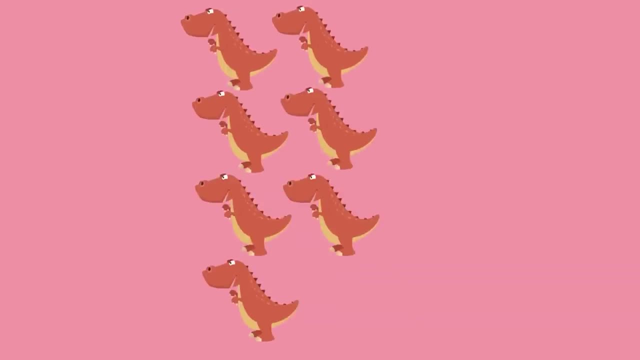 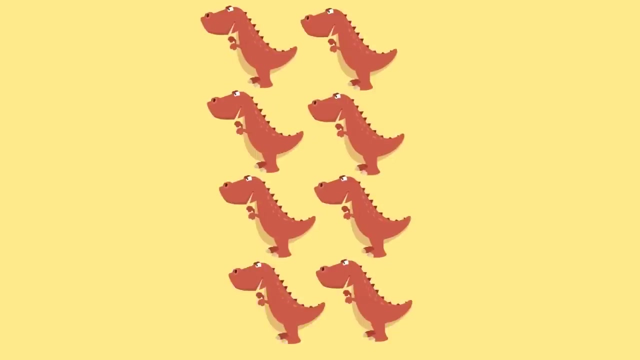 we have seven dinosaurs, but there's one dinosaur that's all alone. six of them have friends, but one is all alone. doesn't have a pair. seven is odd. the number eight does everyone have a friend? yes, there's no one without a friend. number eight is an even number. it splits up into two very nicely. eight is even. 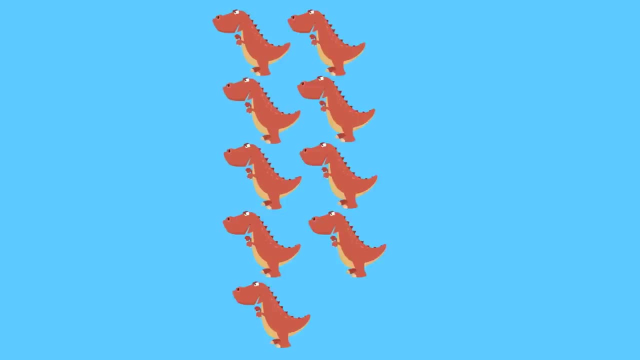 let's go even higher than number nine. now you can see really quick, it's easy to spot: is nine even or odd? yes, it's odd. there's one who doesn't have a friend. nine is odd. oh my goodness. 10, 10, is it even or is it odd? you tell me, you know how to do it now. you know the. 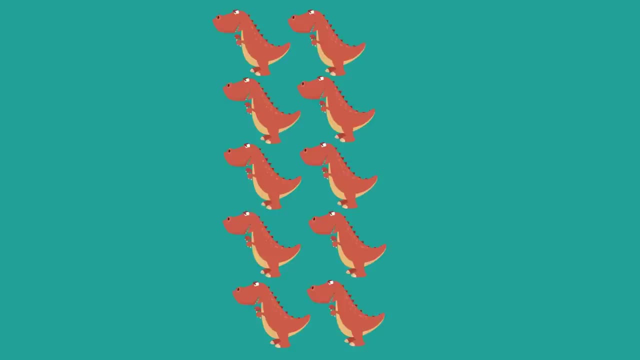 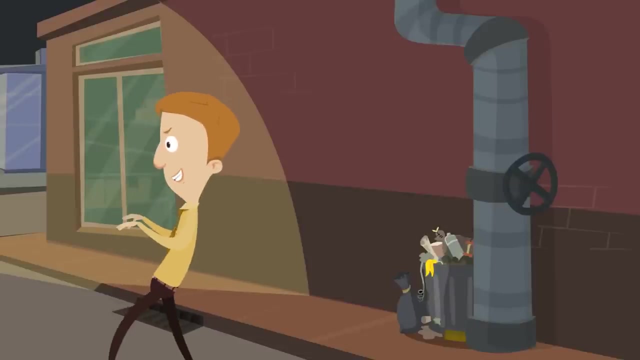 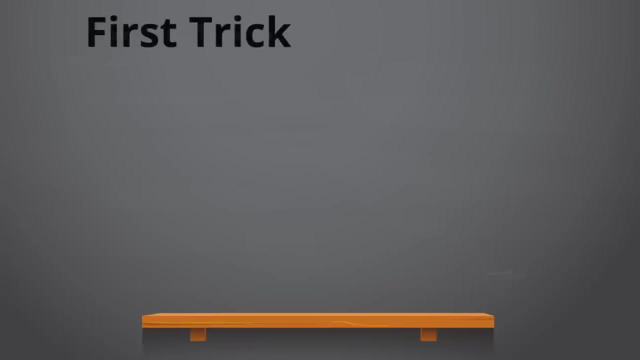 trick. yes, 10 is even. everybody has a friend. now we're about to teach you two sneaky tricks that you can use with even and odd numbers. okay, so seriously, it's well, it's not. it's not really sneaky anyway. so this first trick is that all of the numbers alternate from odd to even, and 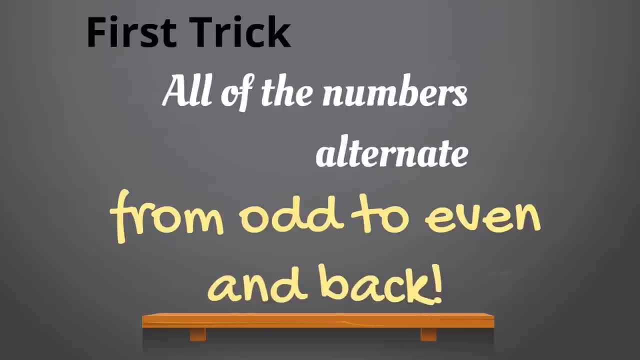 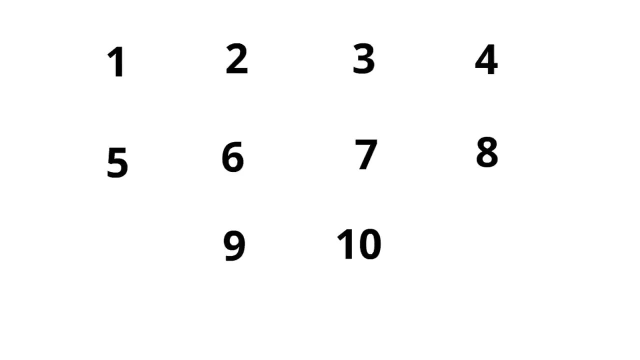 back and we're gonna show you what that means and what that looks like. here we have the first 10 numbers, numbers 1 through 10, and the trick was: all of the numbers alternate from odd to even and back. do you remember? if number one is? 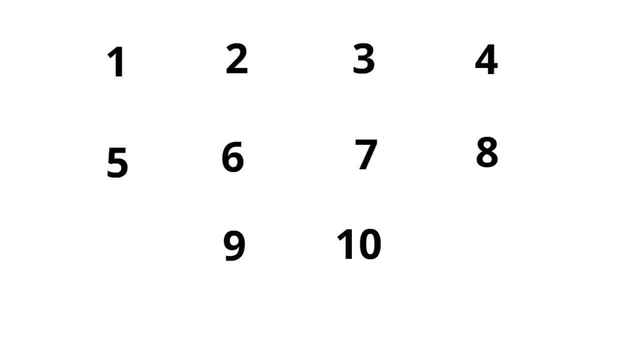 odd or even yes. number one is odd because, remember, number one's, all by himself, doesn't have a friend, doesn't have a partner. it's not an even number. number one is odd. now we remember number two, right. number two is even yes, because it can be grouped in. 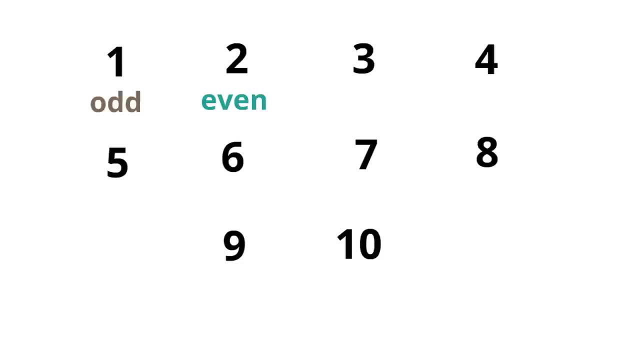 two, because it is two. now if they alternate, that means which one is number three? it's odd. this is where it gets fun. if three is odd, then that means four is even good job, and if four is even, that means five must be odd, yeah, and if five is odd, that. 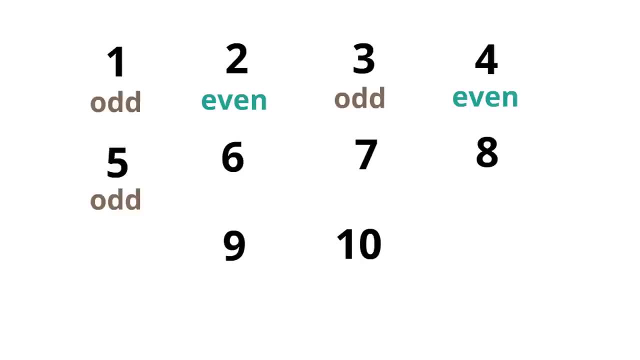 means six must be- you guessed it- even. and if six is even, that means seven must be odd. yes, seven is odd. if seven is odd, that means eight is. come on, what's the pattern? eight is even. and if eight is even, that means nine must be odd. and if nine is odd, come on, is. 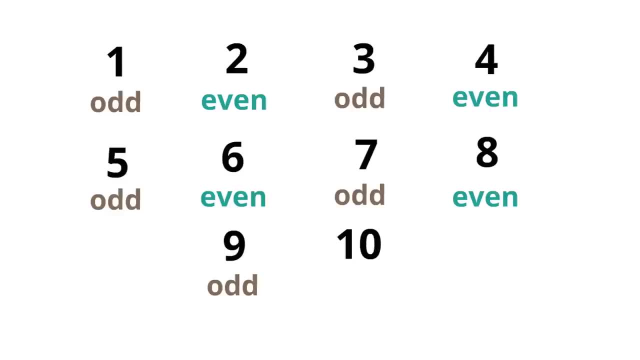 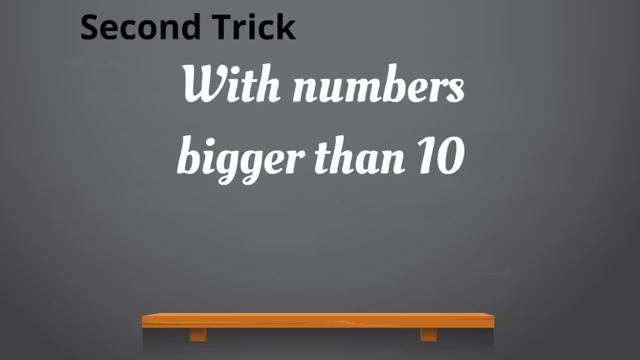 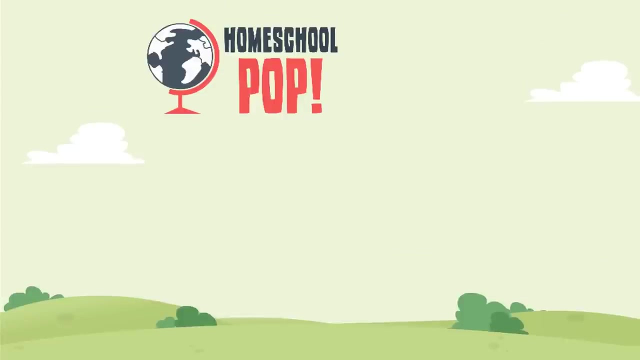 than ten if it's odd. or even you can see on the end with numbers bigger than ten if it's odd. or even you can see on the end to demonstrate, let's play a game we here at homeschool pop call odd, or even we're gonna look. 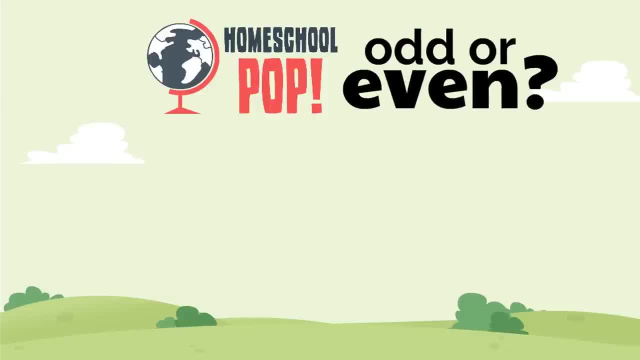 at a number that's bigger than ten. we're gonna look on the end to see if it's even or if it's odd. our first one is the number 21. is it odd or is it even? it's odd how? why? well, we look on the. 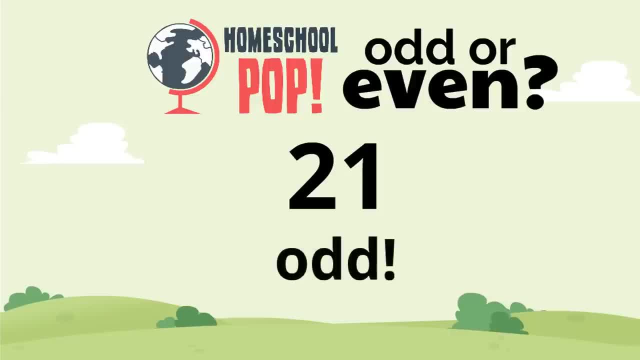 end. the end is a one. one is odd, it's all by itself a 1 is odd. so 21 is odd because one is the ending. did you know? that means 71 is odd and 100 and 1 is odd and 131 is odd and the number 1001 is odd. 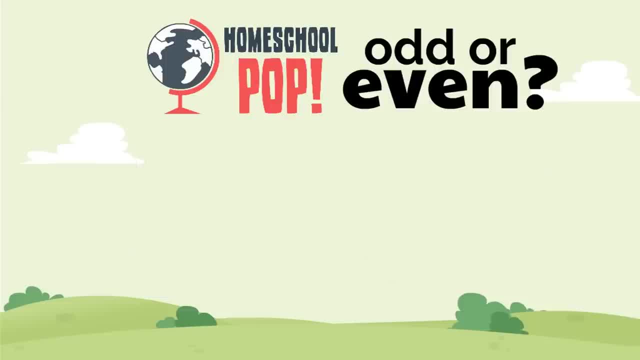 why they all end in one. let's try this one. the number 30 is odd, so fifty here, 32.. Is it odd or is it even? 32 is even. Well, how do we know? Because of the ending. Look at the ending. It's the number 2.. 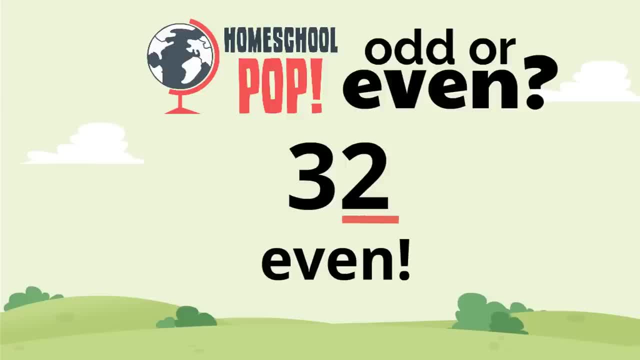 2 is an even number because it's a group of 2.. It can be put in groups of 2 because it is 2.. The same rule applies- This is the second trick- With numbers bigger than 10, if it's odd or even. 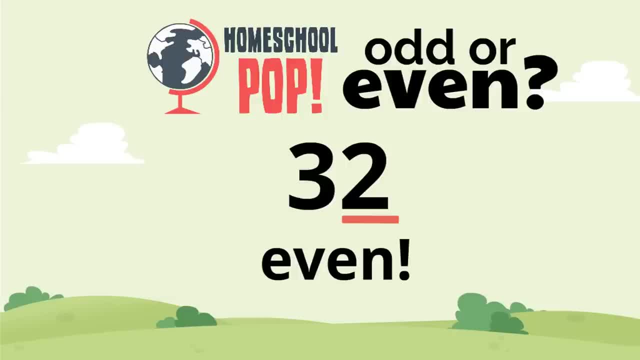 you can see on the end, every single number that you can think of ends in. 2 is an even number. Let's try one. that's a little more tricky. Let's try the number 100.. Is 100 odd or is it even? 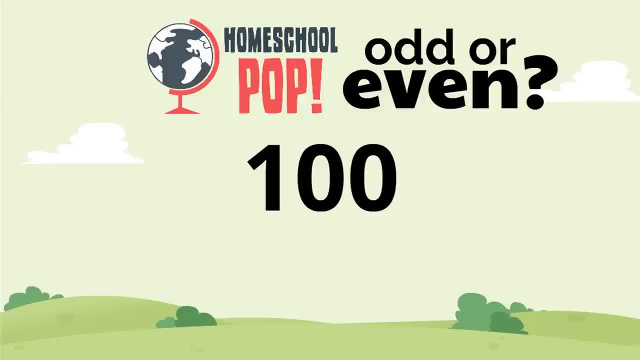 100 is even. It's even and we know that because of the ending It ends in a 0.. Now remember our second trick: With numbers bigger than 10, if it's odd, or even you can see on the end, an ending is a 0 and every number that ends in 0 is even. Let's look at the chart again. 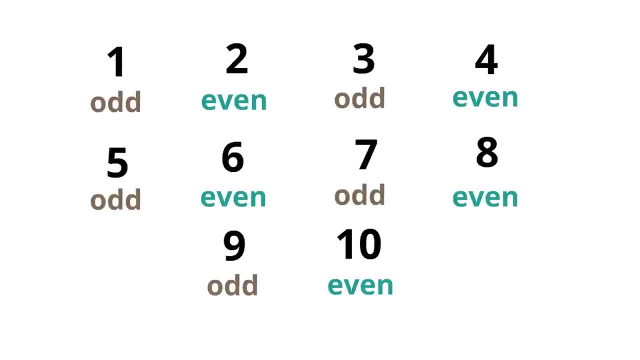 As you can see, 10 on the bottom ends in 0.. 0 is even. Every single number that ends in 0 is even, just like every number that ends in a 1 is odd. Every number that ends in a 2 is even. Every number that ends in a 3 is odd.